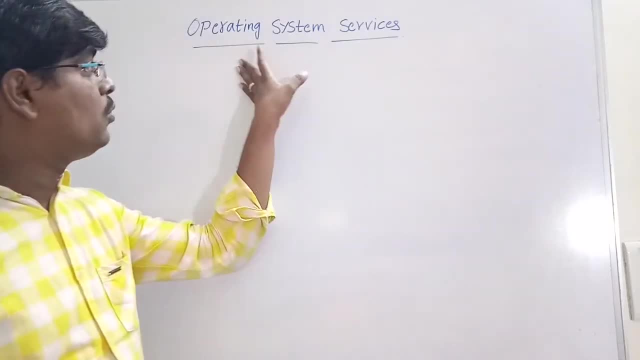 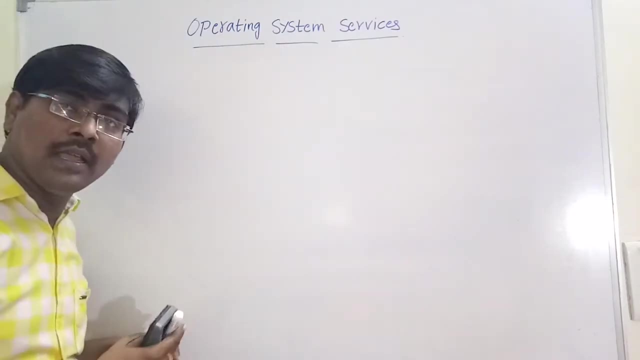 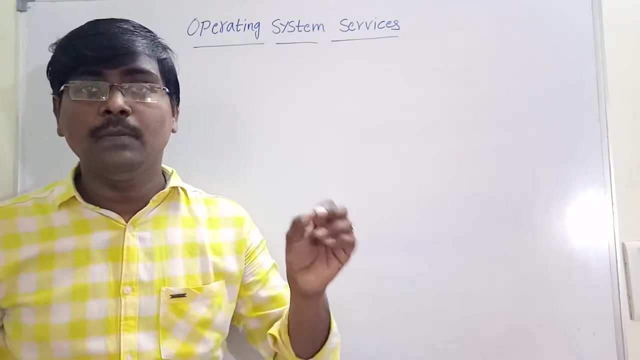 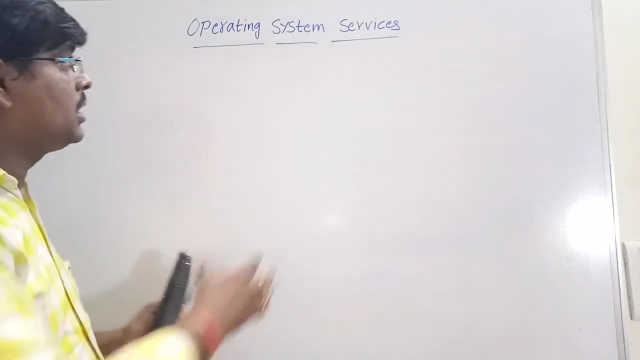 Welcome to our channel. In the previous session we had discussed functions provided by an operating system. Now we will move to the services provided by an operating system. So in the definition we learned how the operating system is viewed. Operating system is viewed in two perspectives, that is, in user point of view and in system point of view. In the similar fashion, operating system provides services to the user and, at the same time, services to the user. 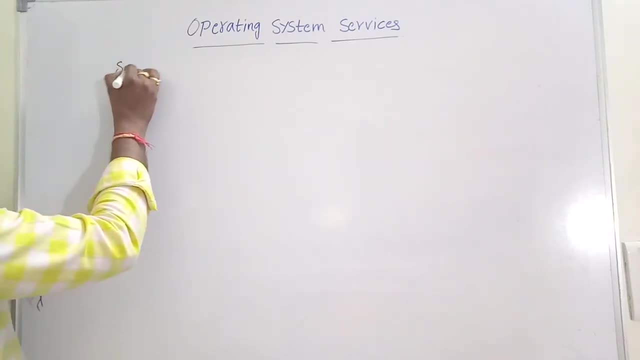 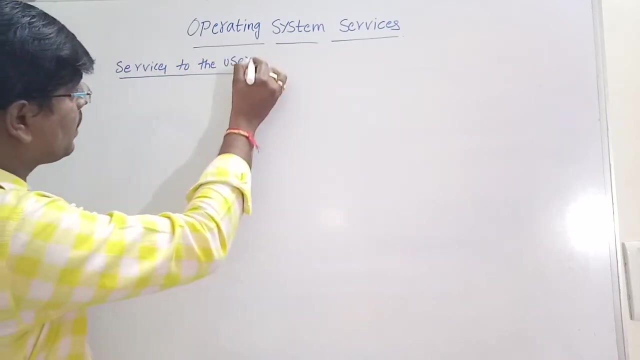 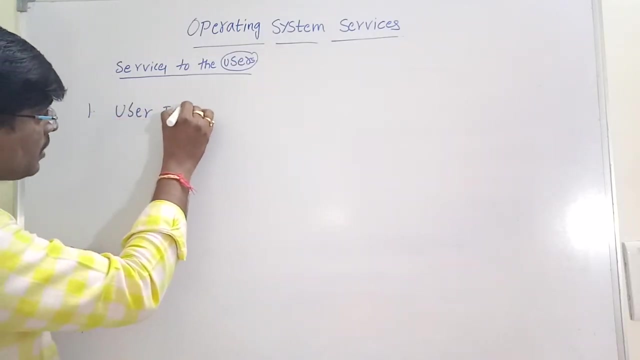 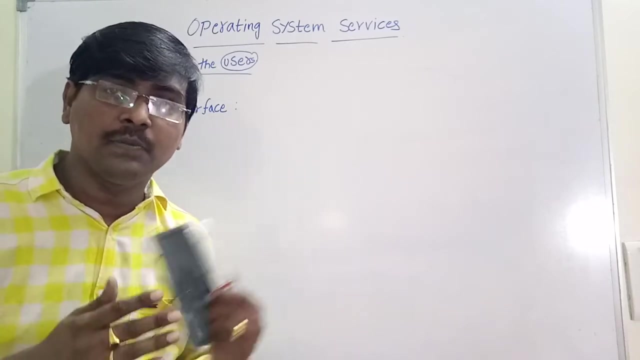 So first we will move the services to the user. What are the services that are provided by the operating system to users? First one is user interface. So the definition itself is operating system is simply an interface between user and computer. So operating system provides an interface to the user. 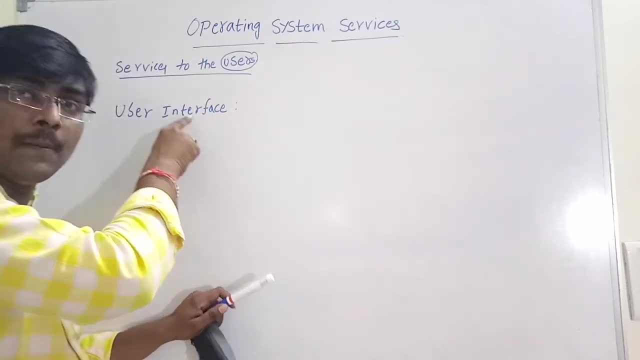 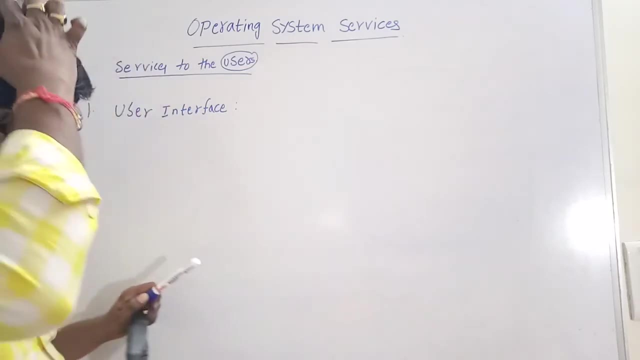 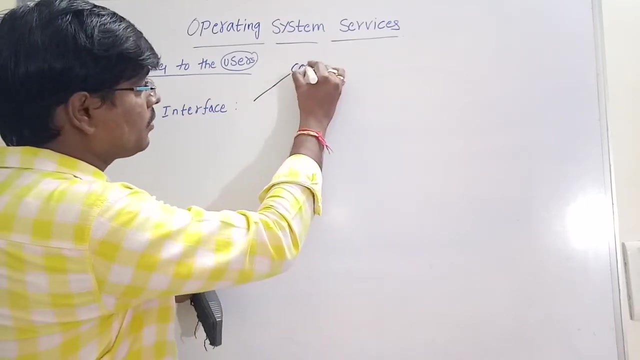 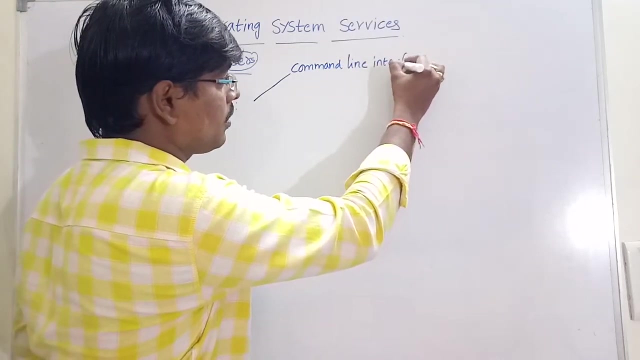 The first two services operating system provides an interface to the user for accessing the computer. For accessing the computer. we have different types of interfaces. We have different types of interfaces. Among them, the first one is command line interface. The first one is command line interface, That means here the existing. 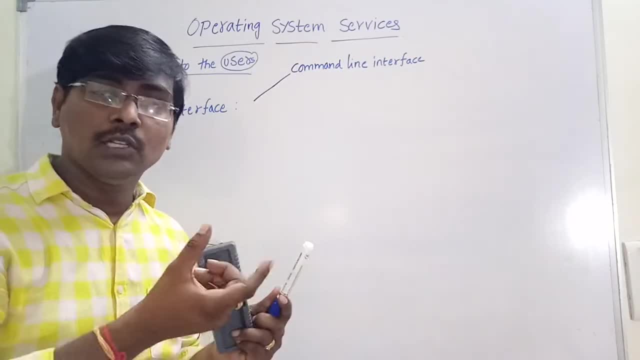 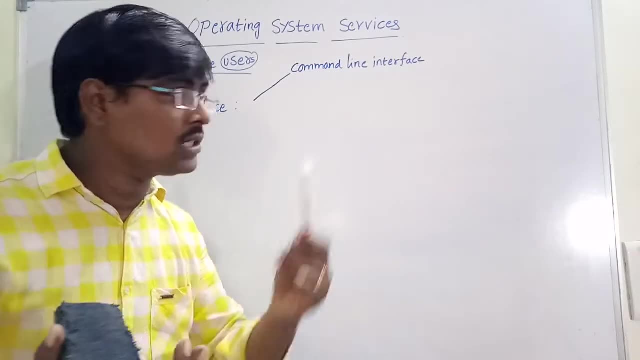 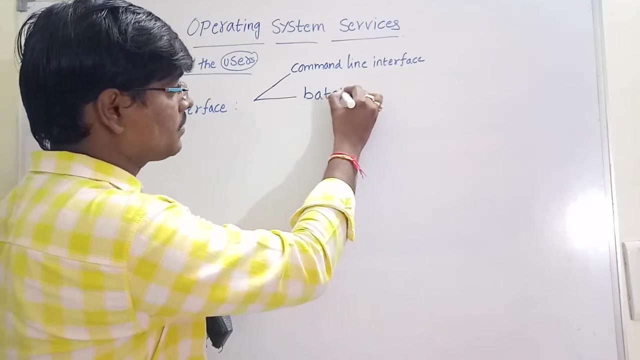 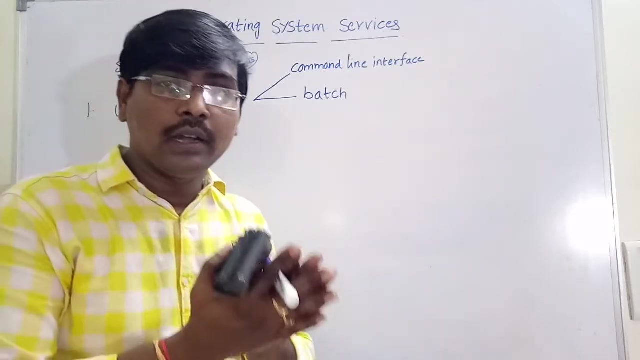 is performed by using commands. Suppose we are opening the command prompt By using those commands, the interface works. That is, we are operating the system by using the commands. And another one is batch interface. Another one is batch interface. Batch interface means the files or the directories are encoded. That is placed in a bag, Placed as a. 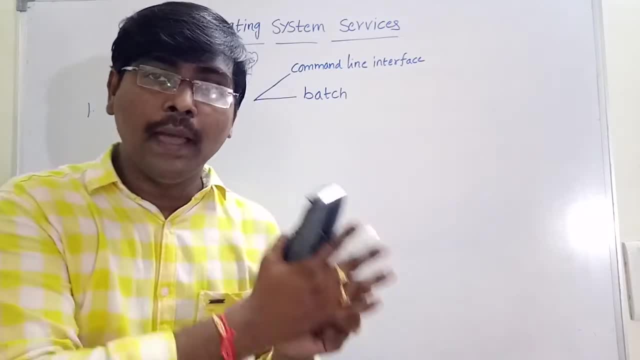 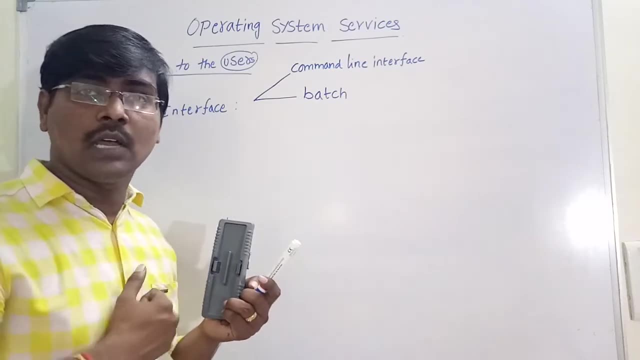 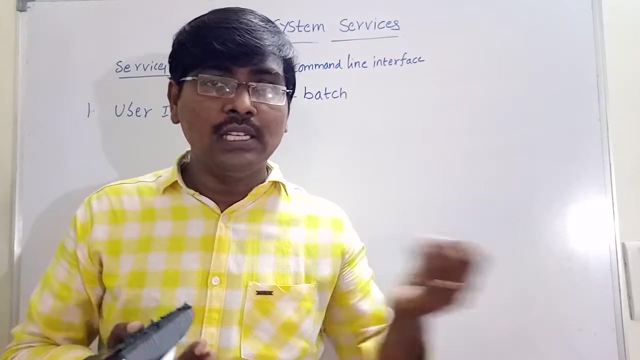 Batch And that batch is executed. One simple example, For example, consider a project. The project contains many number of Java files. Assume Java. The project contains many number of Java files Here. no need to execute each and every file. Simply make a jar file and execute the. 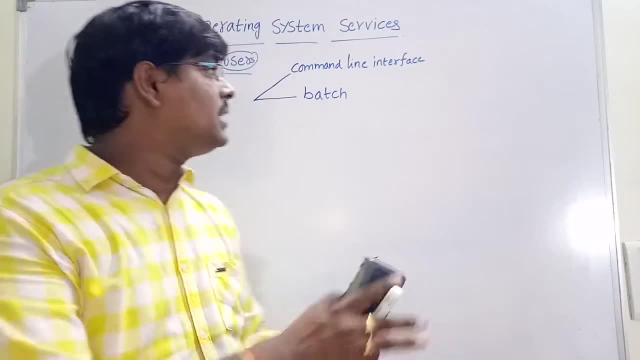 jar file, That is. that is the batch operating system, That is a batch interface means all the files that are needed are like sprinkle dimensions in here or this are like slider, so depress or quality are likeи all the files that are needed are like that is. 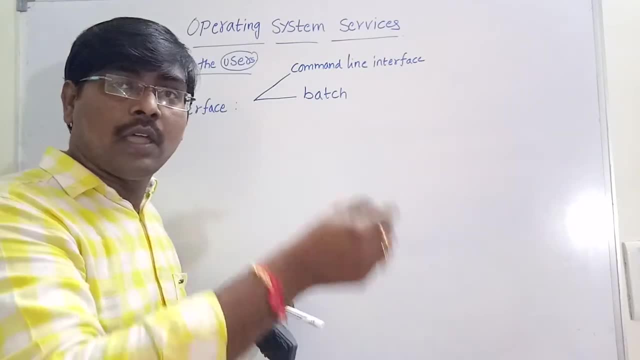 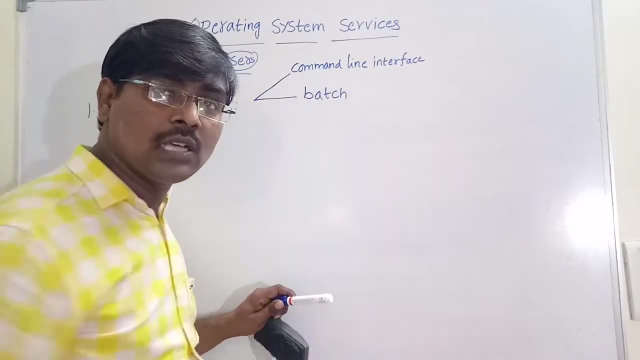 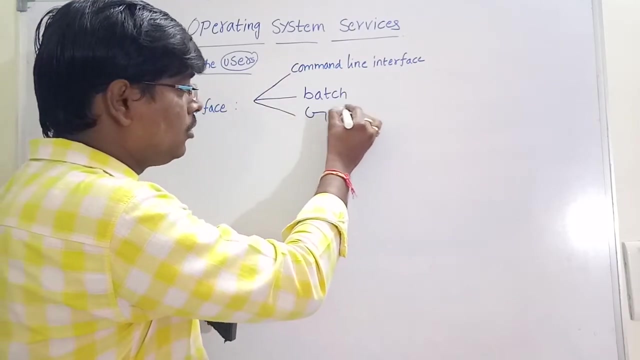 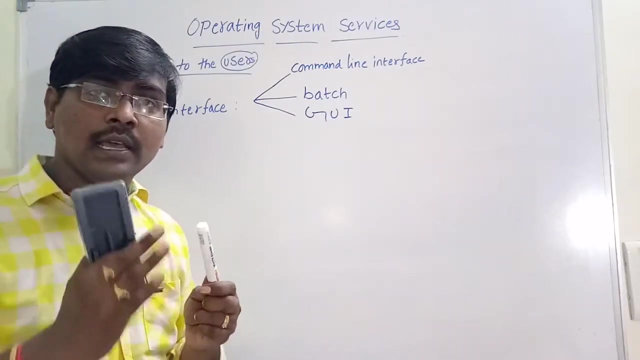 simply the commands and the control over the commands are placed as a batch and that batch is executed in batch operating system. actually, we are not preferring these two. the most likely used one is graphical user interface. graphical user interface- this is the most usually interface. simply graphical user interface provides some pointing devices, that is, pointing some Ivo. 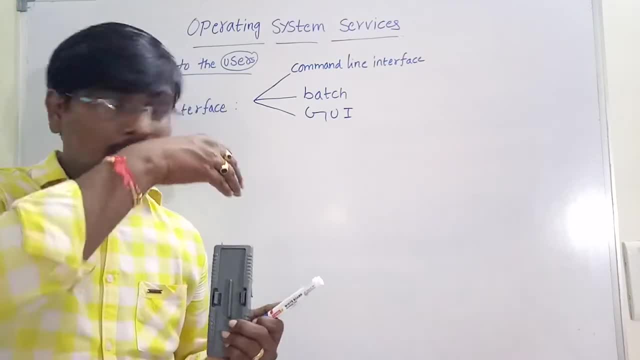 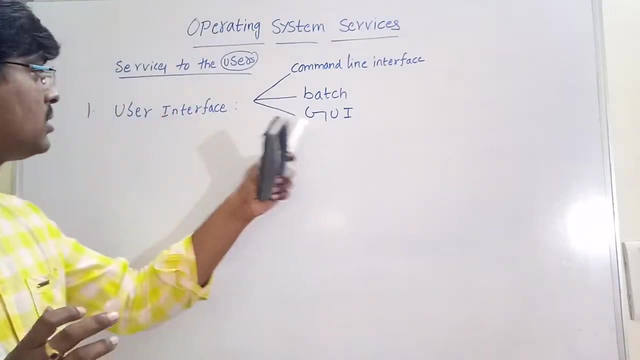 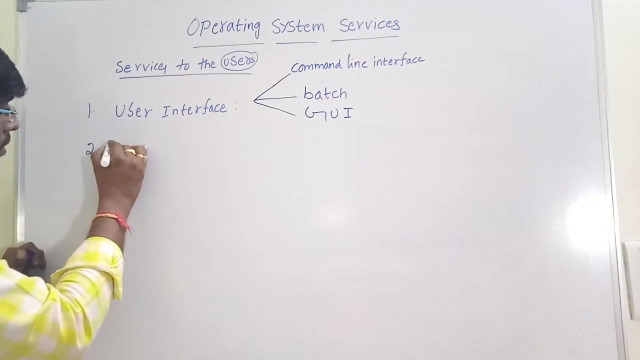 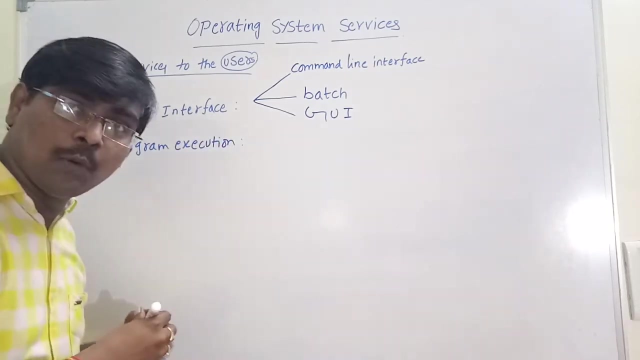 devices to enter the text we are using keyboard and for accessing, for selection, simply by menus and icons. it is very easy. all those services, that is, these are the interface service provided by the operating system. the next one is program execution, that is, if you want to execute a program. 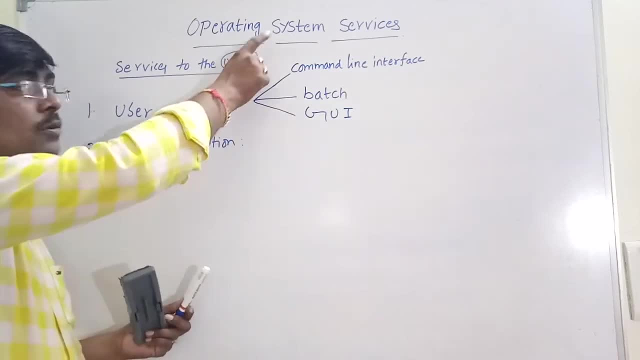 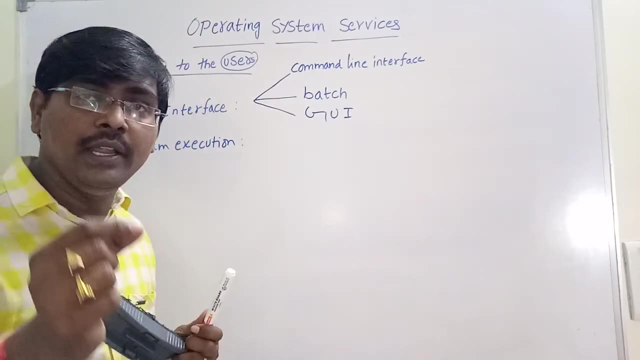 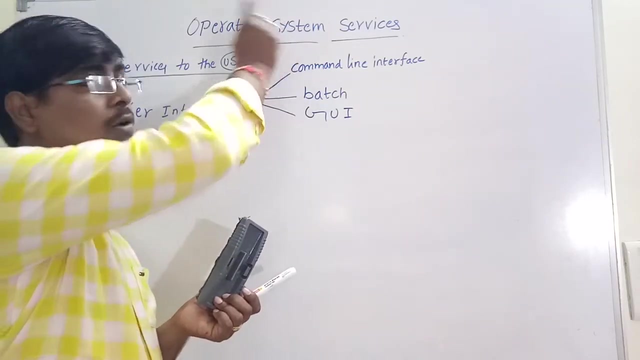 if you want to execute a program, that service is also provided by the operating system. how to execute a program? the program must be loaded into the memory. to execute a program, the program must be loaded into the memory. that is the service provided by the operating system. okay, so during. execution depending on your program. either terminate the program, that is, in the execution time. we can terminate the program either normally or abnormally. that is the second case. so program execution means simply load that program into the memory for execution. that service is also provided by the operating system. so load program into memory. load program into memory for. 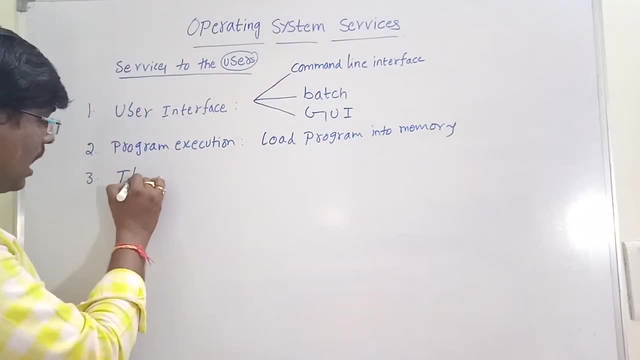 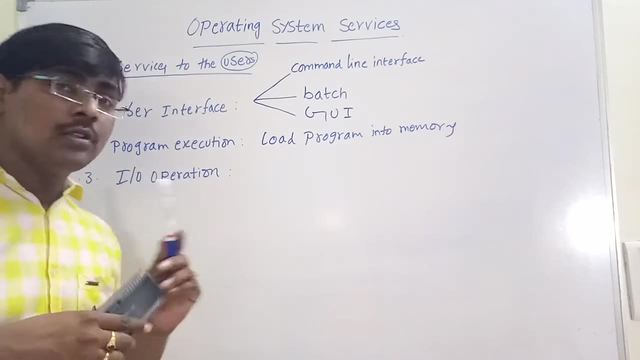 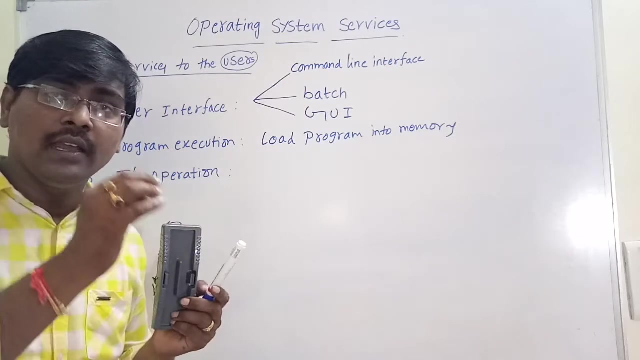 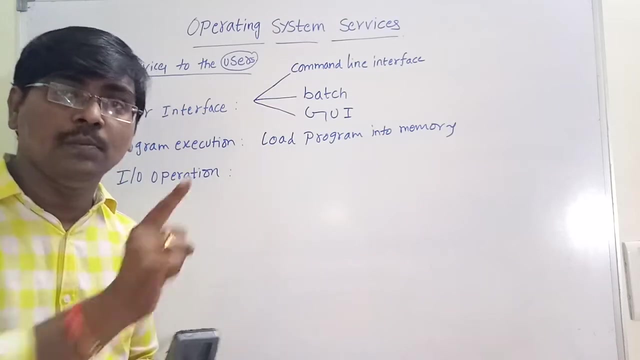 execution. next service is Ivo operation. Ivo means input output, Ivo means input output. so generally users do not interact with the I O devices directly, that is, it is directly not using I O devices. if you want to use I O devices, that is accessed by using operating system only. okay, so no direct use. 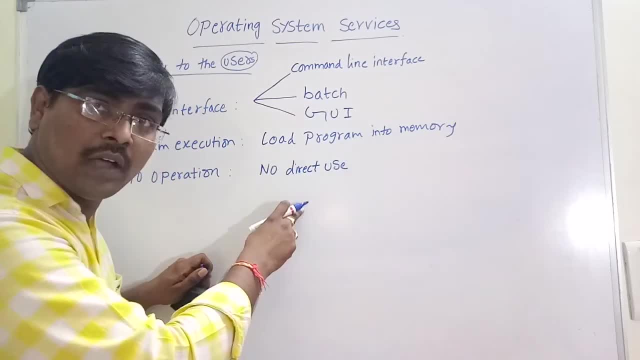 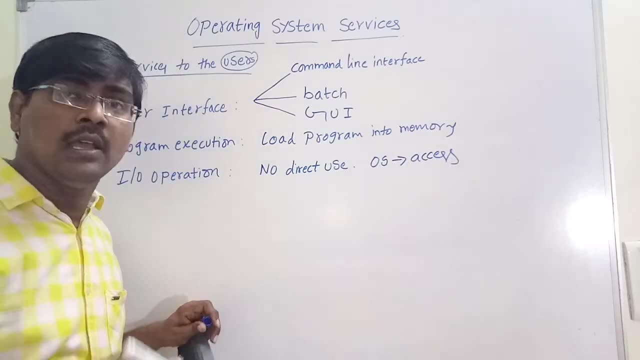 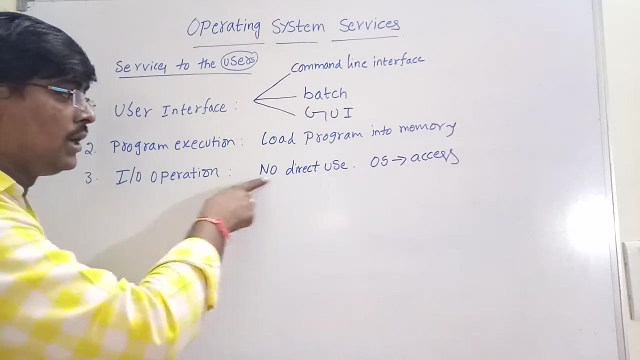 actually there is no direct use of I O devices. so operating system provides the access to the I O devices by using some means, that is, by. operating system follows some technique for accessing of I O devices. okay, remember this one directly: it is not possible to use I O devices without operating system by. 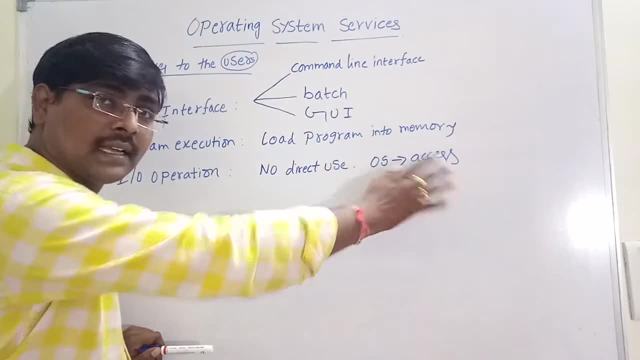 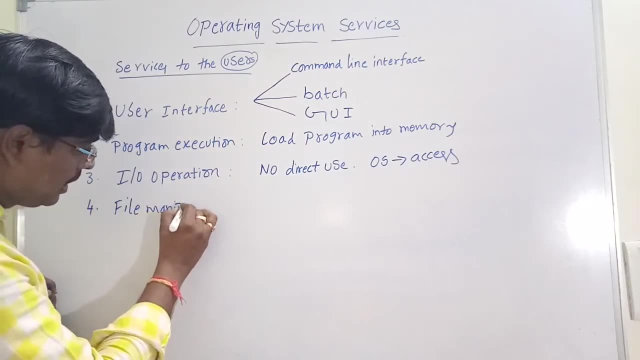 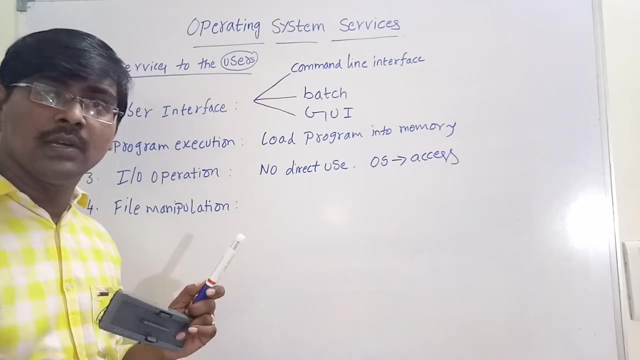 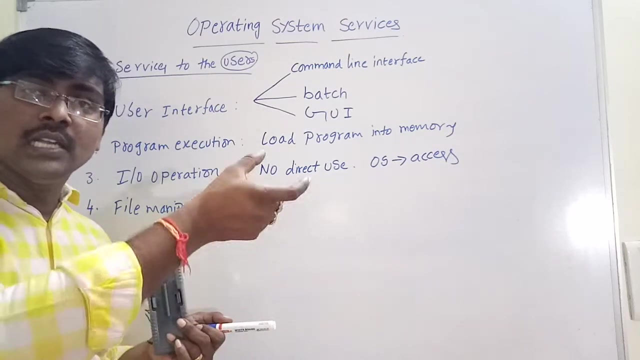 means of some technique operating system provides access to the I O devices and file manipulation. that means reading of your file. that means reading of your file. reading of a file means suppose if your system contains some, what file. if you want to open a file, close a file, read the information in the file. search for a. 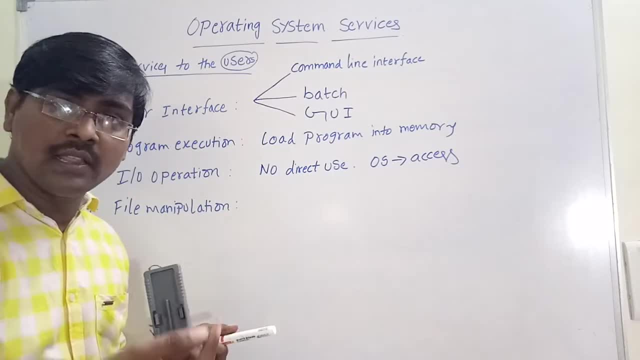 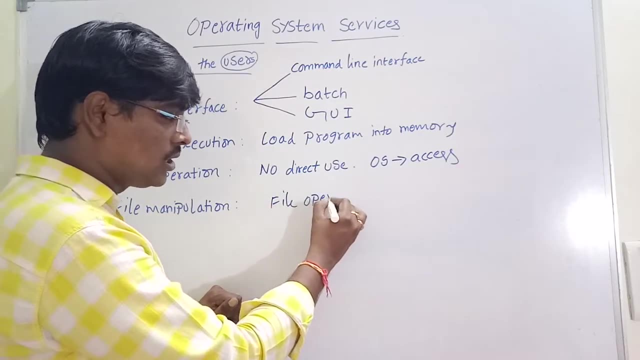 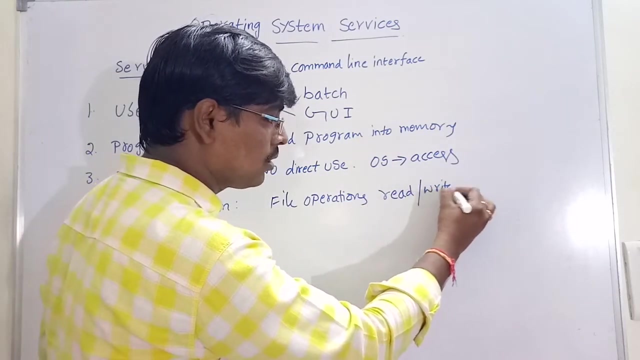 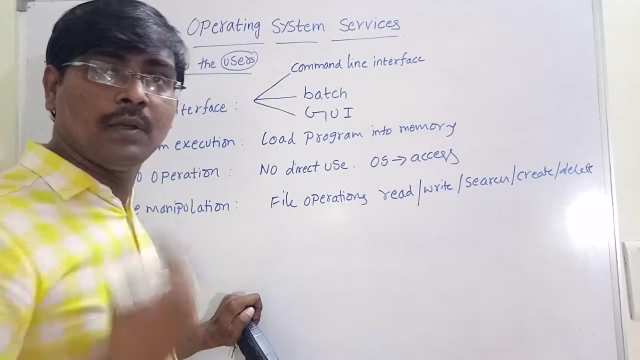 file in the directory by using either name, by using either a content, deletion a file, all those file operations. all those file operations are provided by the operating system. that is simply either read, write, search, create, create a file, delete a file, and so on, etc. any number of operations, all the file. 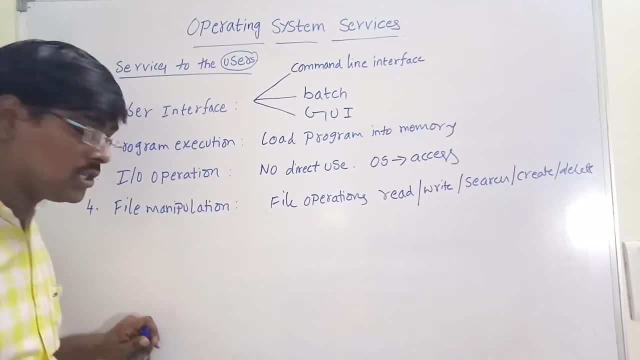 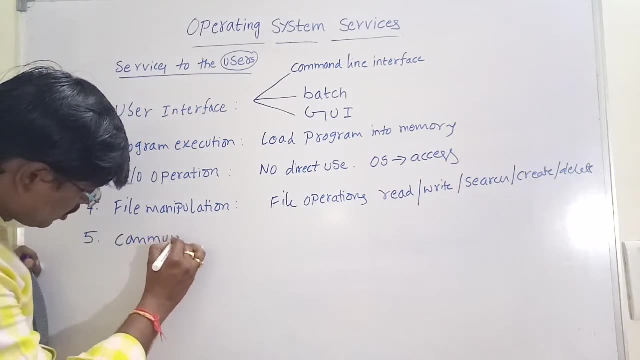 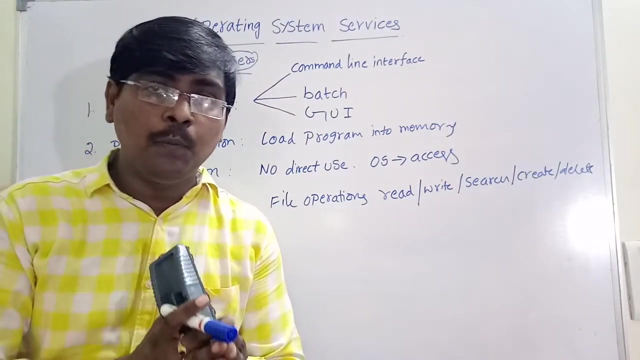 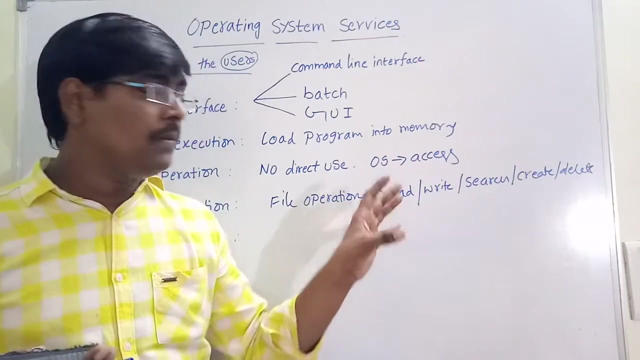 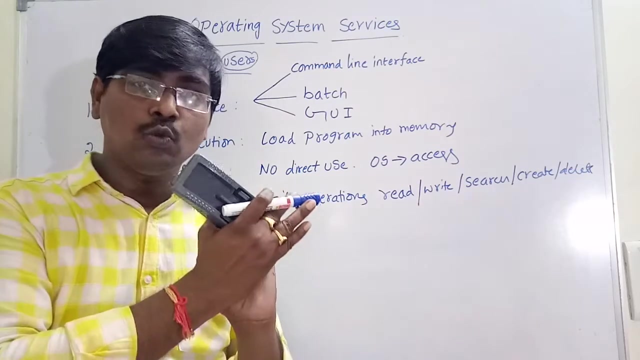 operations are also provided by the operating system communication. communication means suppose during execution, if one process needs to exchange information with another process. if you are using multi programming system, in multi programming system one process needs to exchange information with another system, then compulsory those two process are must be communicated with each other via some communication line. 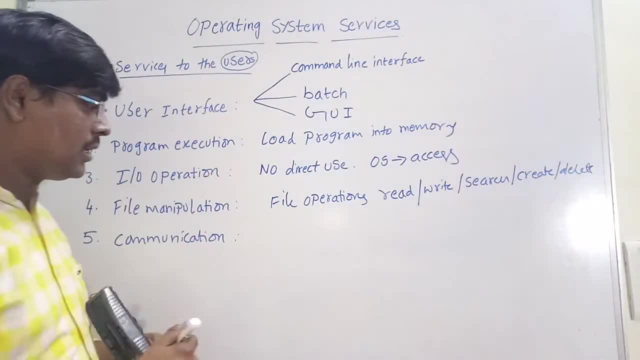 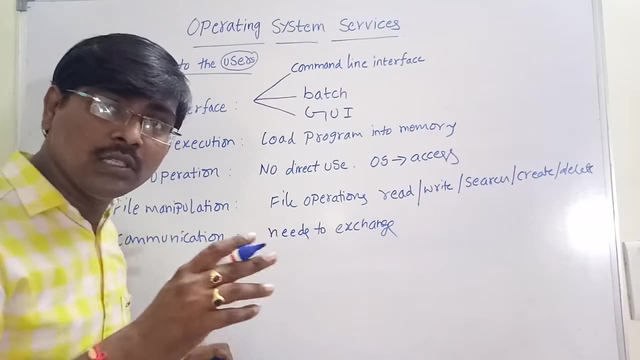 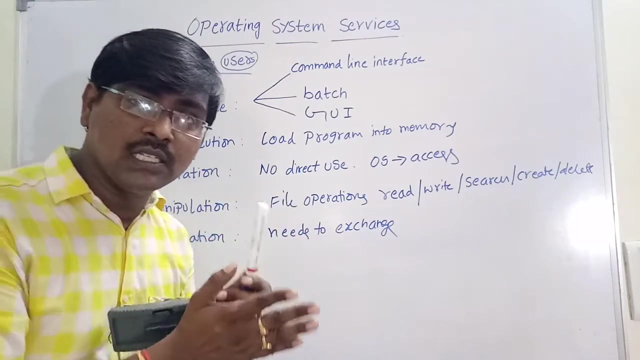 etc. that service is also provided by the operating system. okay, so needs to exchange information if the two process are either in the same system or in the different system. whatever it is, if two process wants to exchange information if the two process are in the same system or the two process are in different systems, that is. 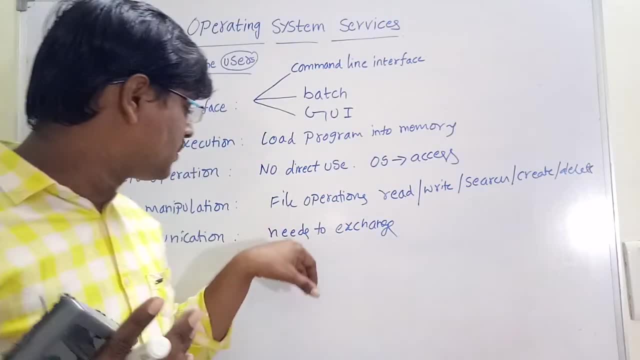 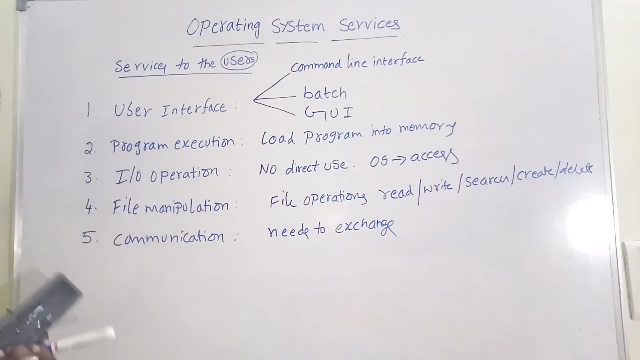 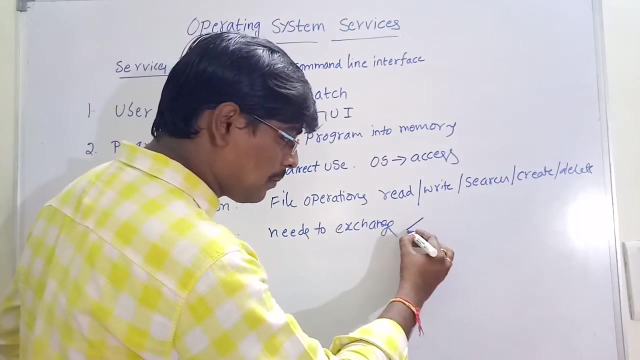 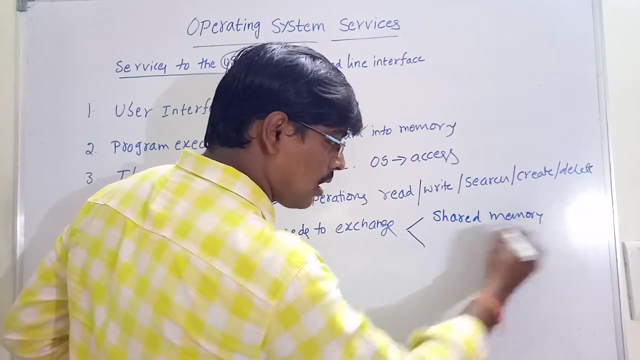 at different terminals. that communication service is provided by the operating system. that service is provided by the operating system. okay, that is communication. that is communication generally. how this communication is implemented. remember, the communication between the processes are implemented by using shared memory or message passing. these are the two. 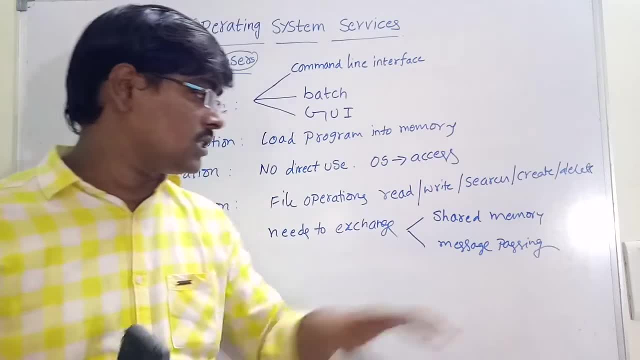 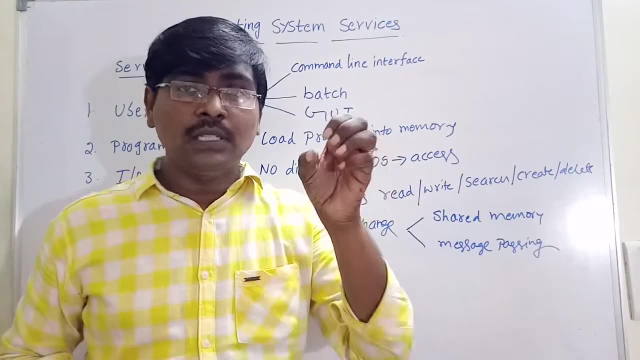 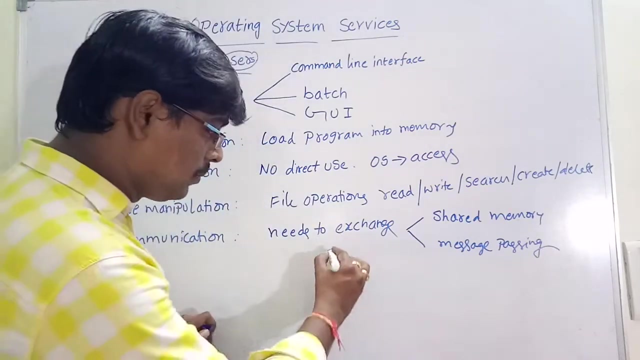 techniques for providing communication between different process, shared memory or message passing. what is mean by shared memory? the operating system maintains a, some section of the memory, that is some part of the memory that is to be shared among multiple process, for example. this is the memory in this I am fixing a. 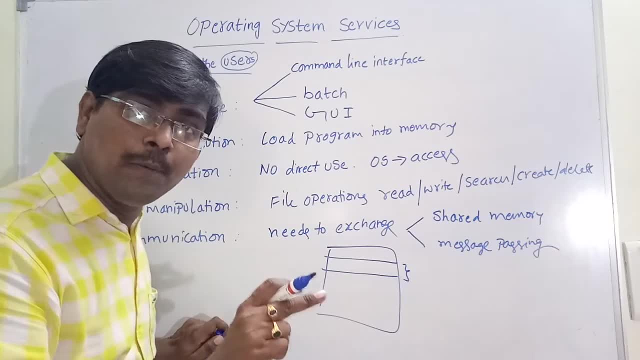 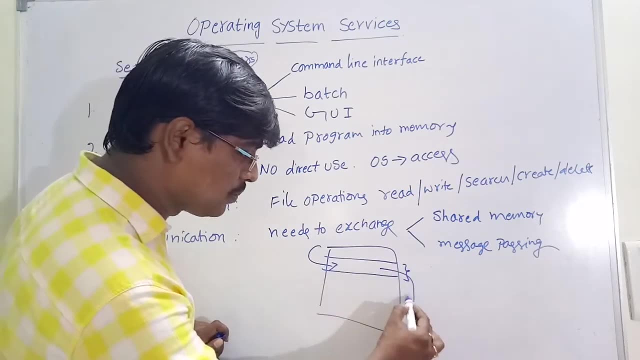 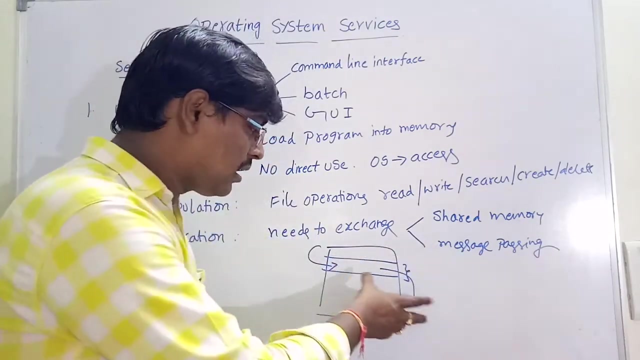 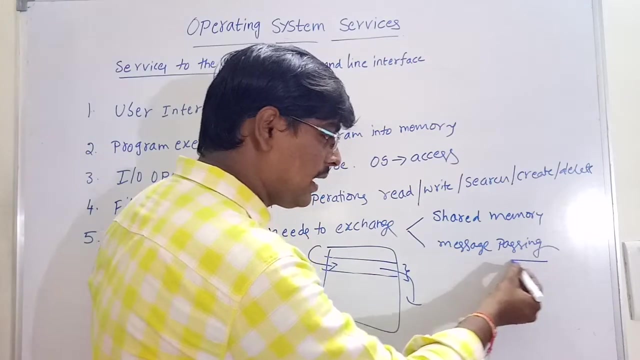 region. suppose this is the shared region. if any process wants to share the information, suppose process P1 places information into the shared region, process P2 access the information from the shared region. this is the way. if any process wants to communicate, they can communicate by using this shared region of memory. shared region of memory, okay, and the 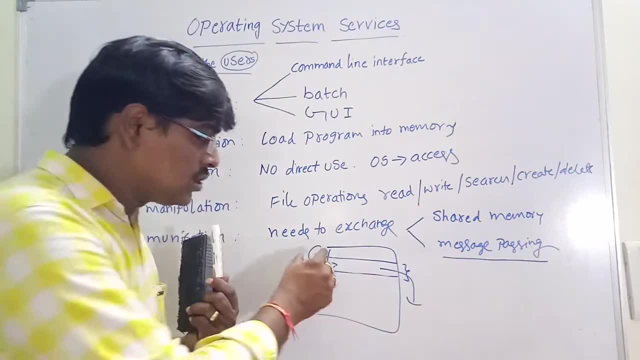 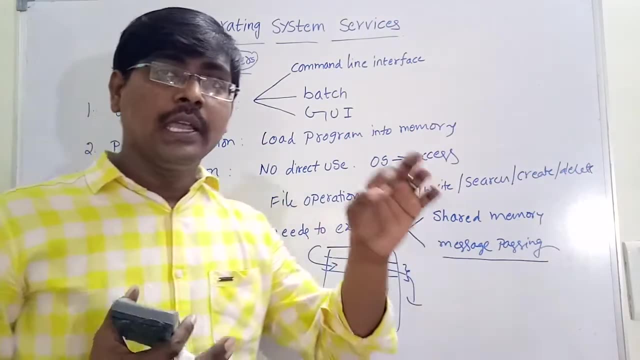 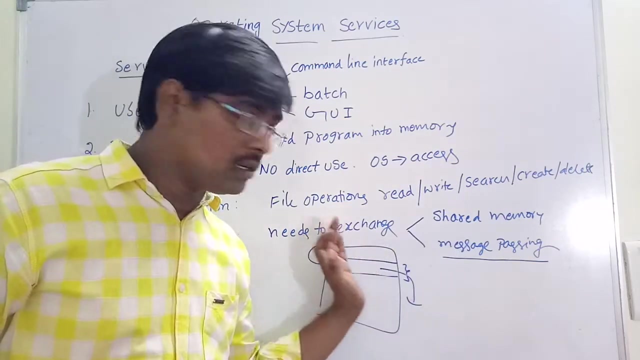 another one is a message passing. that is one process. communicate with the other process through some packet format. that is, information is transferred in some packet format. the structure of the packet format is predefined, so by using packet format we can transfer the information. that is communication, so no. 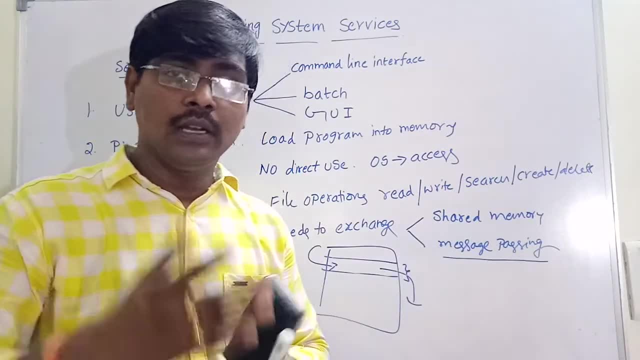 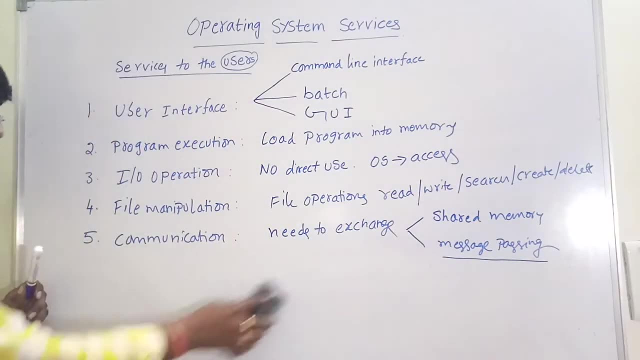 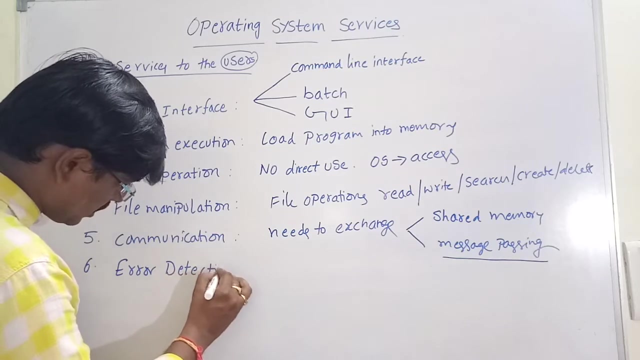 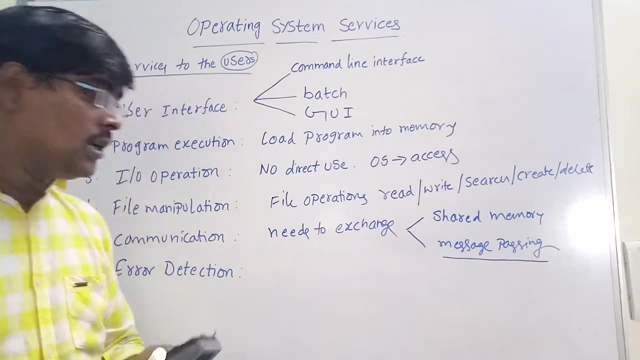 problem. these two concepts are discussed in second part of this video, that is, in inter-process communication. inter-process communication- okay, and finally the error detection. error detection means suppose if the usage of a system, if any error occurs here. error means suppose if you want to use a memory, if the memory is attached. 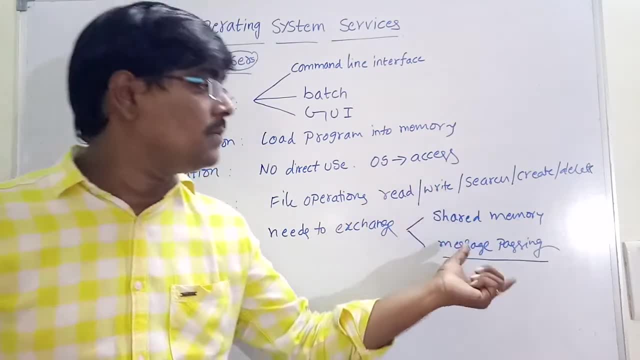 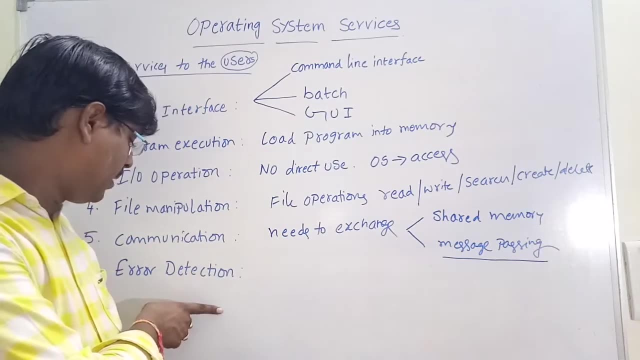 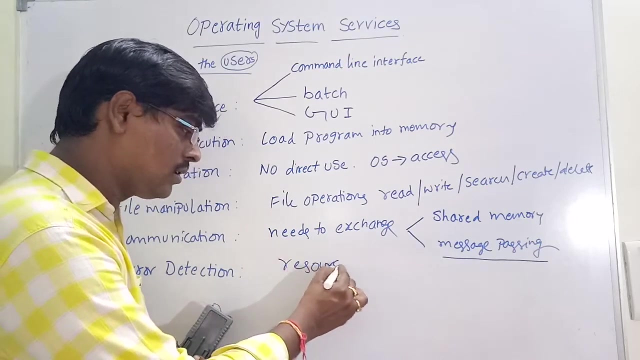 or if you want to use some CPU, if there is a failure in the CPU, if you want to use some mouse, if there is a failure in the mouse. all those resources, errors are identified by the operating system. okay, all the there is a possible errors. all the resources, the errors are identified by the operating. 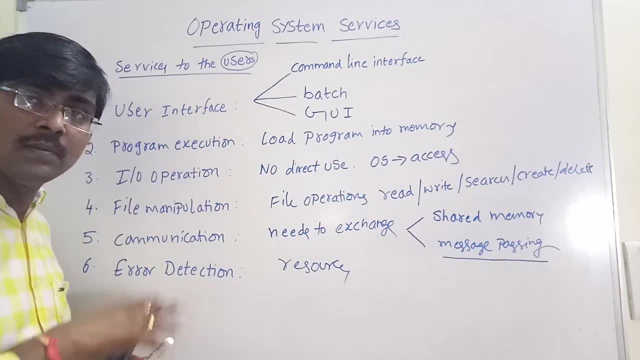 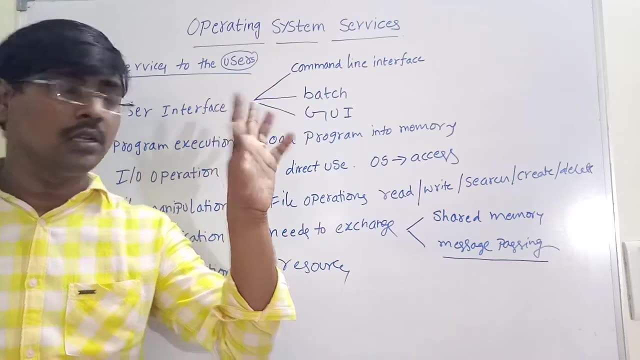 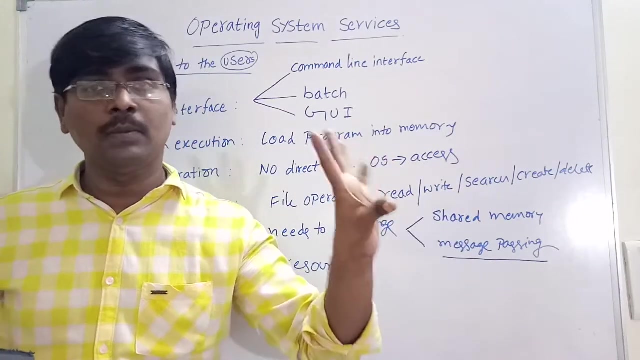 system. these are the services provided by the operating system to the user. simply, whenever you open a system, whenever you open a system, first it displays user interface. so that is one service: after opening the system, if you want to open your file, if you want to open some information, suppose if you. 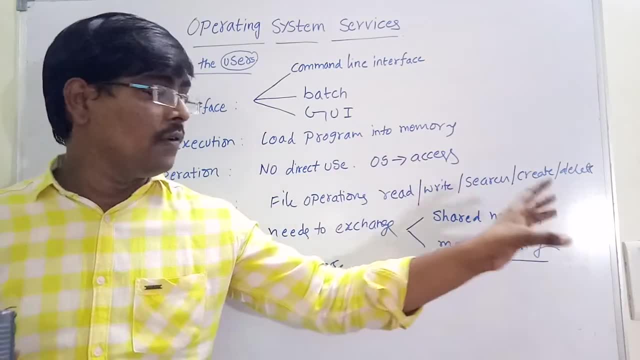 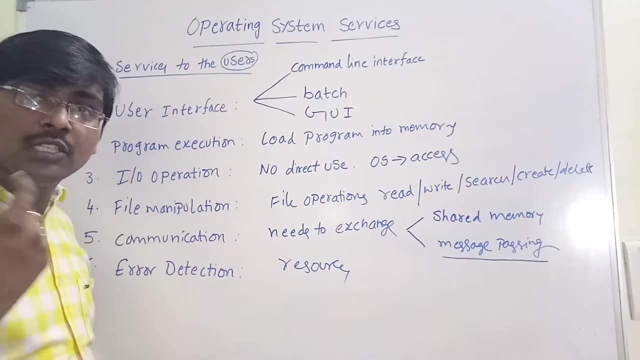 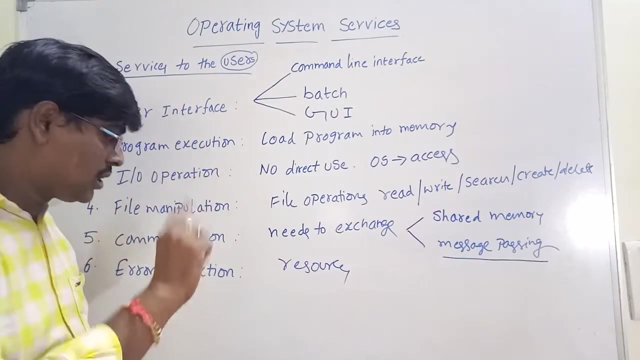 want to open some Google Chrome, that is one operation. if you want to open some particular file you want on laptop, that is your file. that is one service. you want to open, execute a program. if you want to click some icon, I have operation execution. so if you want to share information from one person to another, 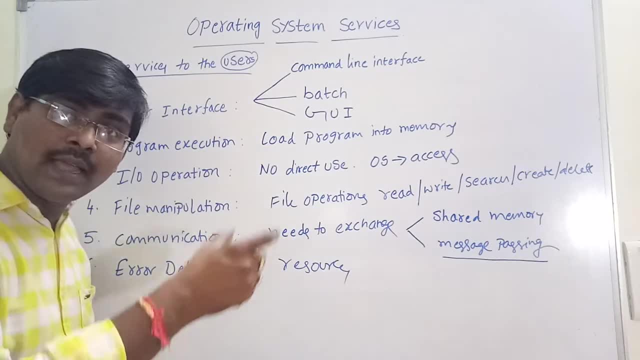 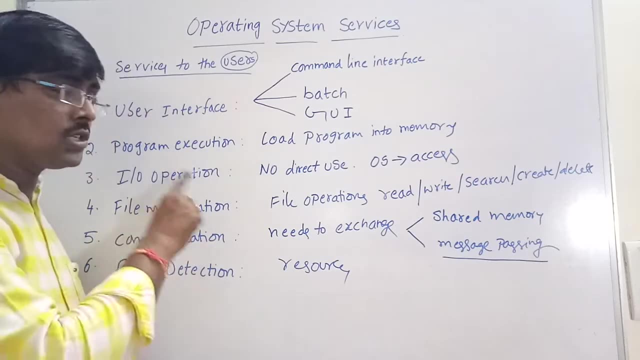 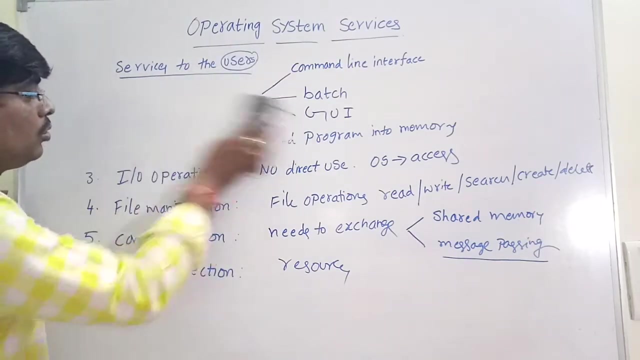 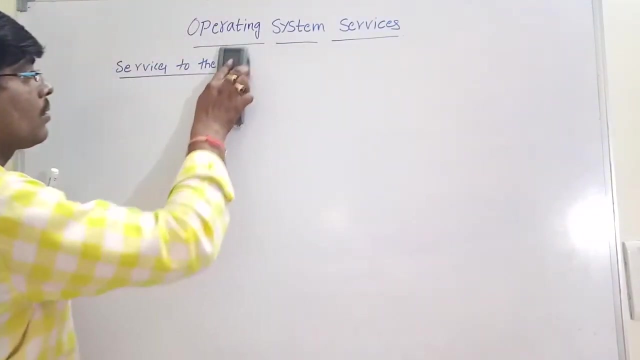 person. so communication if there is any error for accessing some information, that is error detection, all those services. these services are provided by the operating system to the user. okay, now we will discuss the services provided by the operating system to system, services to the system. what are the first two service? the first two service is resource allocation. resource allocation. suppose in multiprogramming. in multiprogramming that means multiple number of processes, request for a resource, multiple number of process request for a resource. the resources are allocated by the allocated by the operating system. Okay, where multiple programming means multiple number of programs in the system, for all the programs the operating system has to allocate. 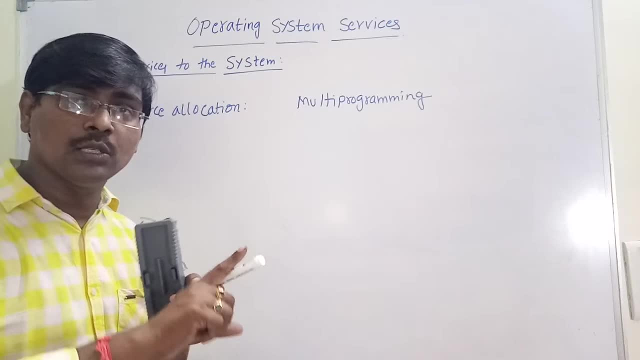 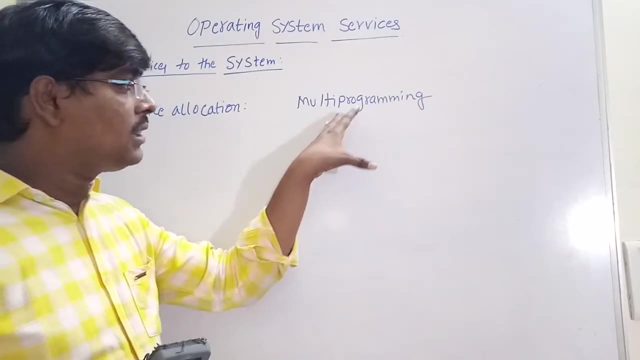 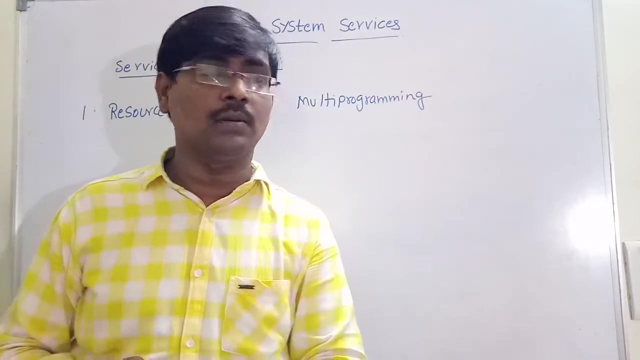 the resource. here, resource means CPU is a resource, memory is a recess file device. Everything is a resource. Ivo device is a resource. So, depending on the requirement of the process, the operating system allocates the resources to each and every process in the system, Each and every process in the system. Okay, Next one is. 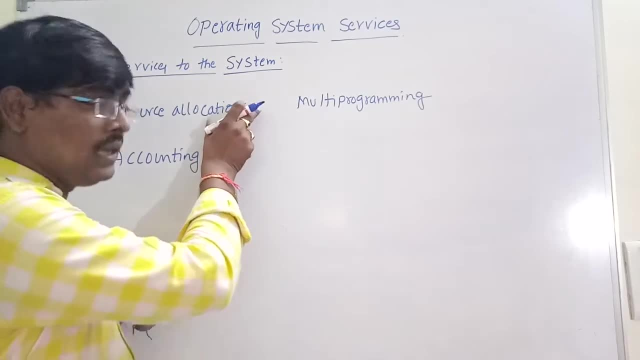 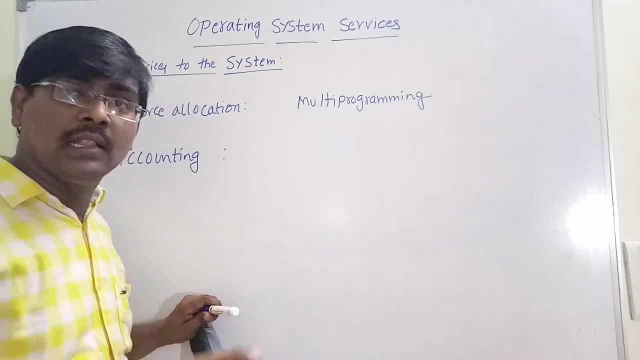 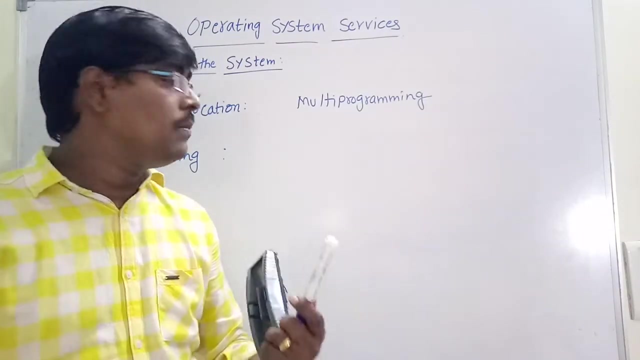 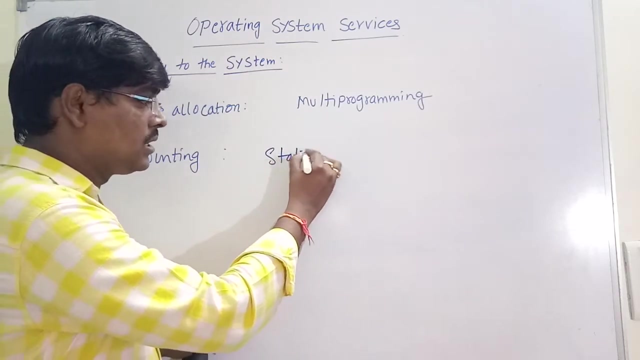 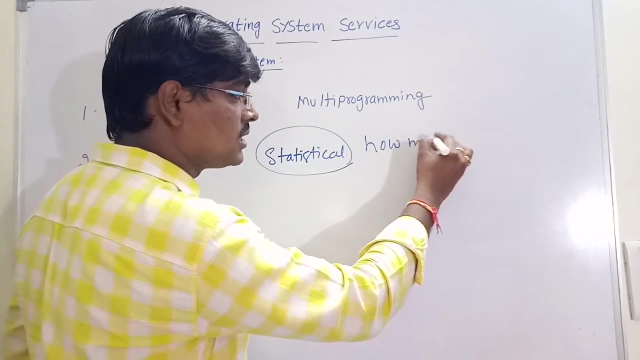 accounting. So simply, in resource allocation, How the resources are allocated. Whenever the resource is free, then only it is allocated. how the operating system know whether the resources is free or the resources Is allocated. simply, the operating system maintain some statistical information. operating system maintains Some statistical information of all the resources. That means how much amount of resource is allocated. 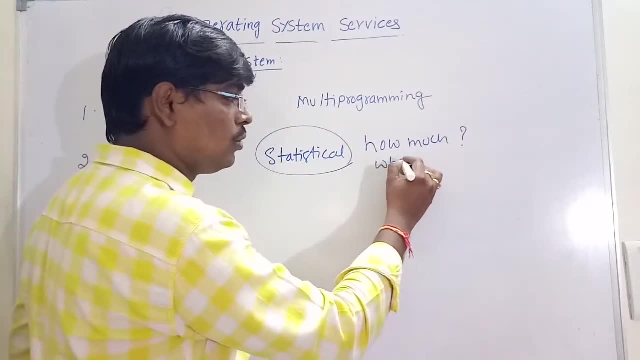 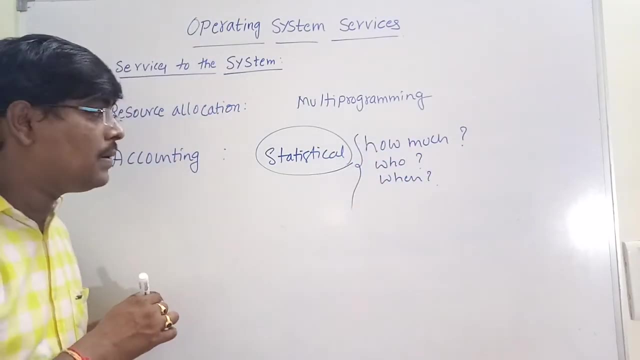 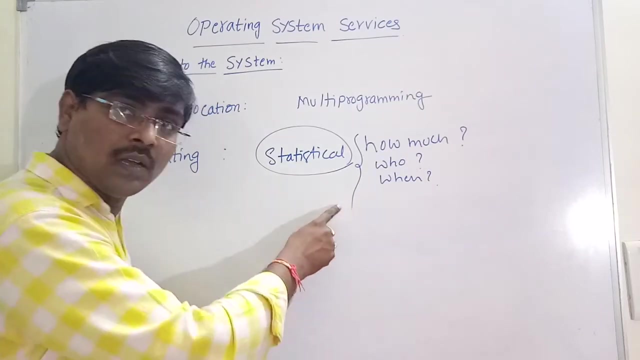 How much amount of resource is allocated, for who we are allocating the resources. Even we are allocating the resources. all those information is maintained based on this information. Suppose, if a process request for a 500 bytes of memory, Check this statistical information: whether 500 bytes of memory is available or not.